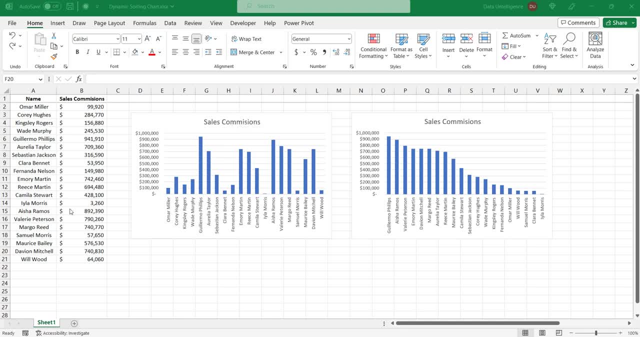 comes up in this way Just displays exactly what's in the table in the same order. But what some people like to do, and what I personally like to do, is just have a little bit more of a visually pleasing display by sorting those sales commissions from highest to lowest. 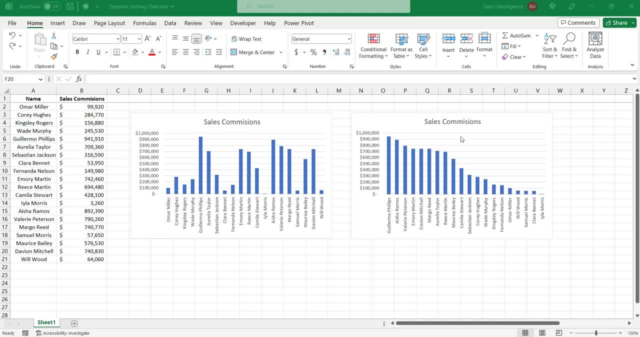 And I want this to be dynamic, so if things change in this table it's automatically going to update the chart on the right hand side. So, for example, we've got Clara Bennett here and if we change her sales value from $50,000 to say $1.2 million, she'd now be the highest. 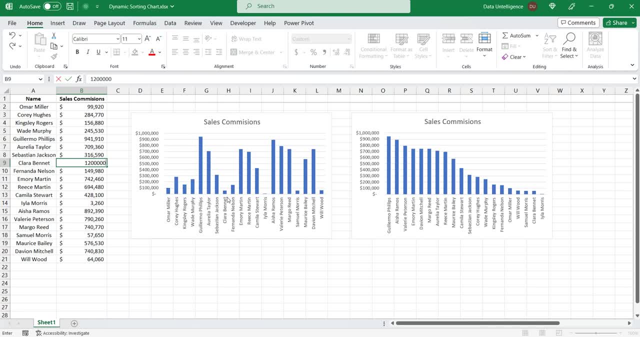 sales person in that list On the original chart. it will change, it will update, but it won't change the order and it won't do anything else. dynamic. But on the right hand side the chart she'll also be allocated that $1.2 million in sales. It's going to re-sort this. 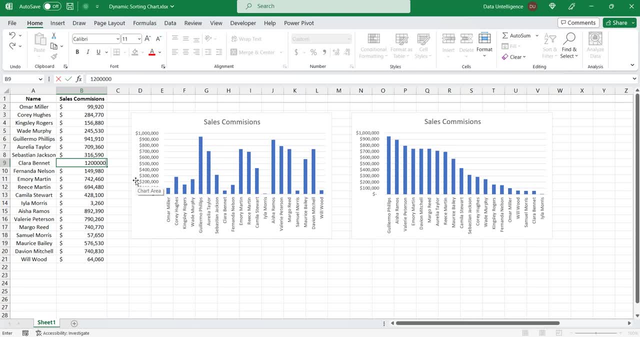 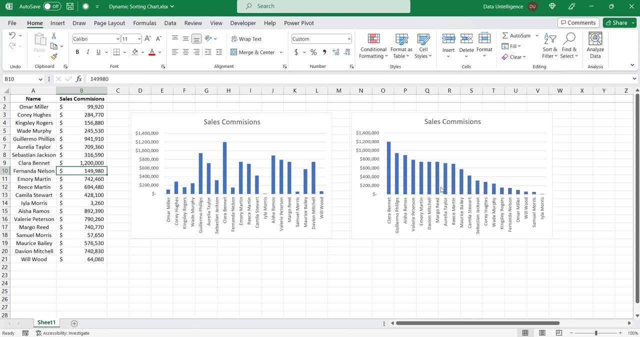 chart and bring Clara to the top of the list. So let's press enter there and you can see that's done, It's re-sorted. it's dynamically sorted, this chart on the right hand side. So it's a really simple process and I just want to show you how to do this in a couple 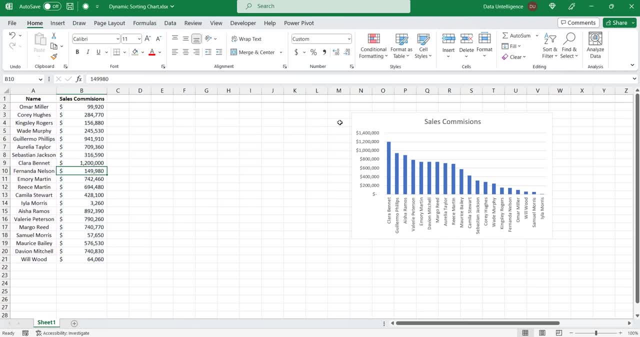 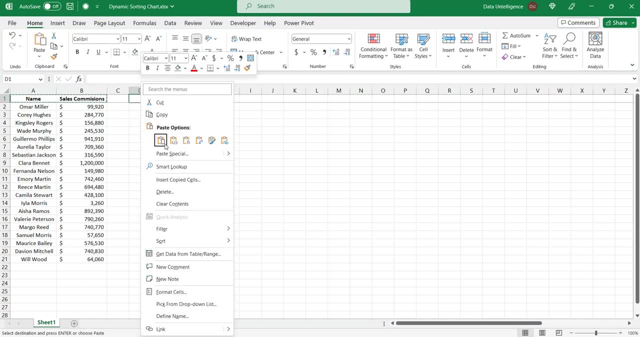 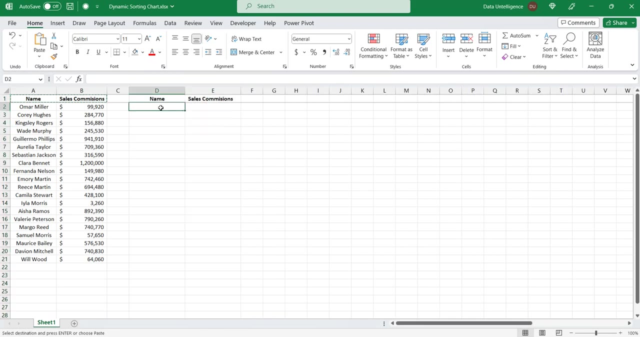 of easy steps. So let's delete these charts and I'll show you what to do. So I'm just going to create a new table, Copy Paste, Just make these a little bit wider, And now I'm going to use the sort function. 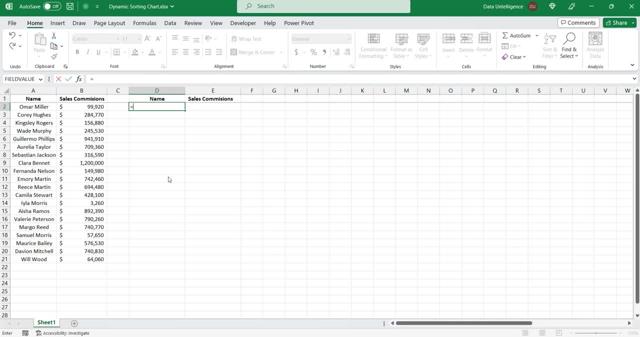 Very easy function to use: Equals, Sort Open brackets. Now, what am I sorting? I'm sorting this table here, So I've selected the cells that I want to sort. Press comma: The sort index is: which column am I sorting? Now? in this instance, there's only two columns, so 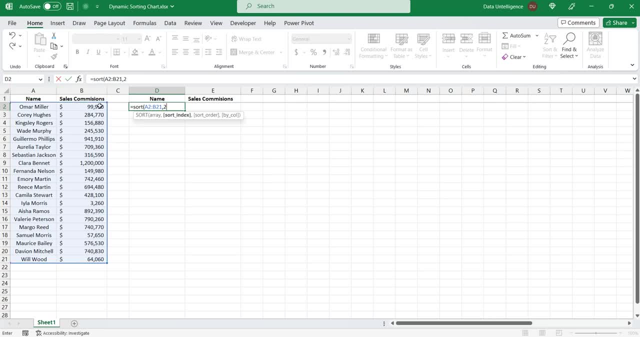 I'm going to sort the second column, Column number Number two Comma And the sort order. If I type in one, it's going to sort it by smallest to largest. If I type in negative one, it's going to sort by largest to smallest. So let's. 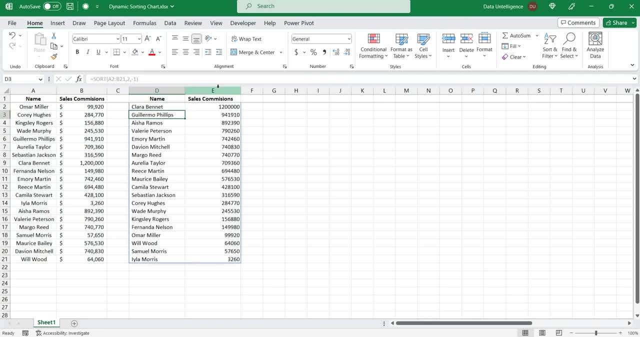 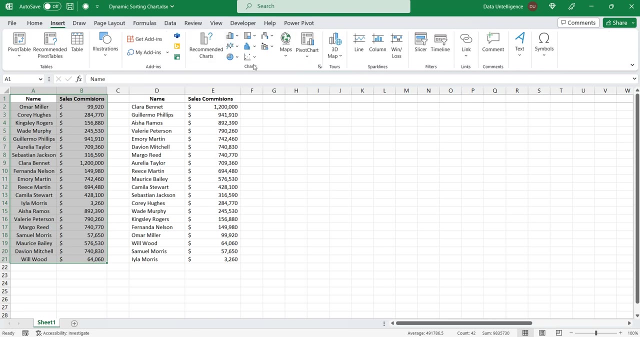 type in negative one And press enter. And now you can see. the sales values are sorted in order Highest to lowest. Now, if I create this chart now, typically what I'd usually do is I'd select the cell range, Insert, Go up to charts.